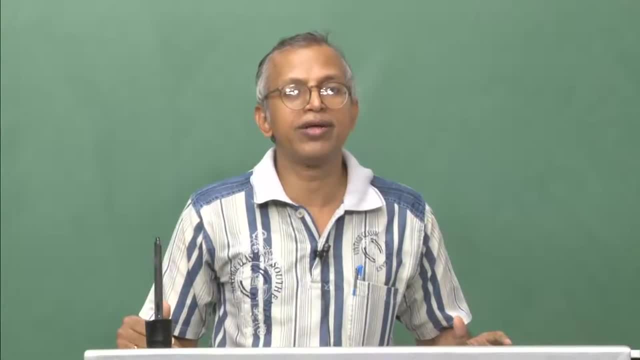 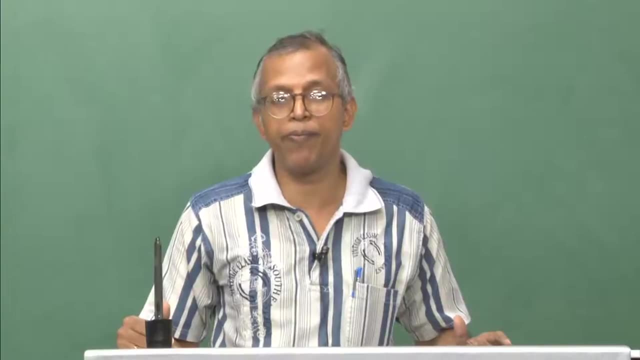 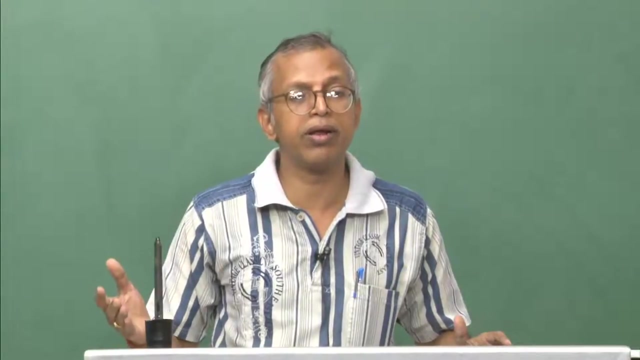 Of course, before that we derived the Bernoulli's equation for compressible flow and also the incompressible flow, and generally the Bernoulli's equation for compressible flow is, you know, being used, but it cannot really be used for the compressible flow. and then we moved into 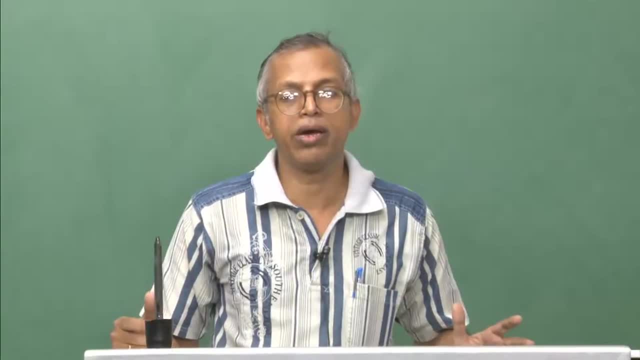 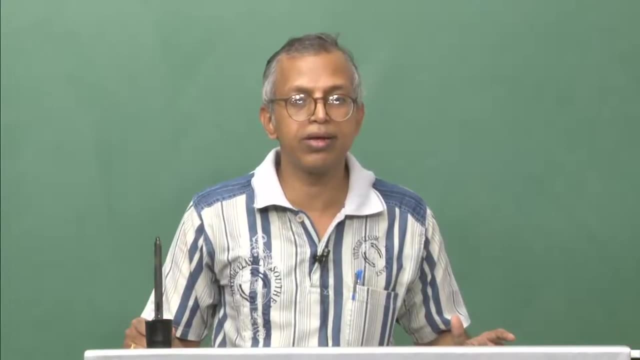 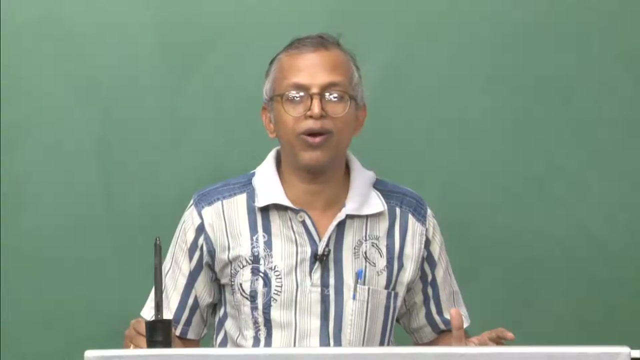 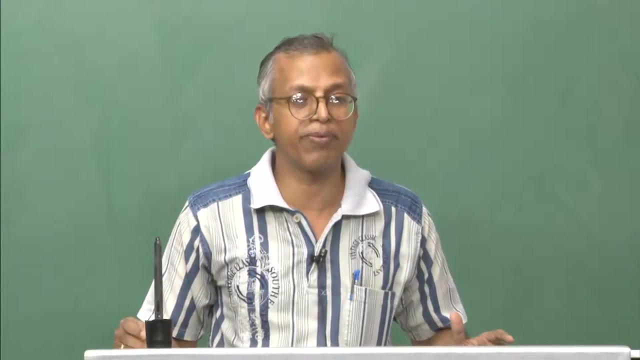 isentropic flow Where there will be no dissipation. that means no change in entropy and also it will be adiabatic. So I guess you might have thought about the question I had asked in the last lecture, that why really we will have to look at isentropic flow, which is quite restrictive in nature. 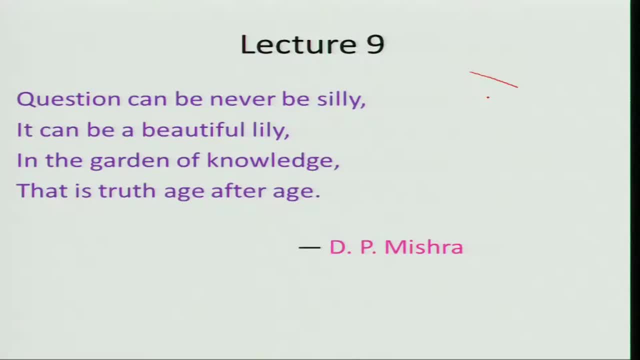 can anybody tell me why it is so? Let us consider a flow in a converging duct. what we have seen. let us say there is a flow which is coming over here and what will happen? it will increases because there is a change in what you call velocity between the station 1 and station 2.. 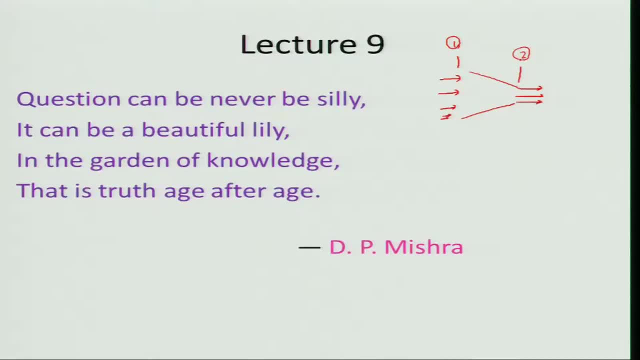 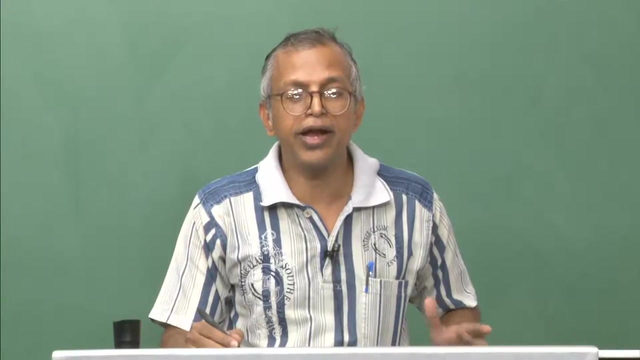 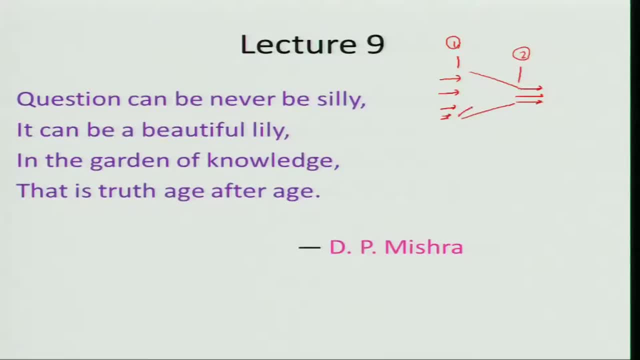 So friction will be there, what you call in boundary layer, here somewhere right, and unfortunately I have drawn a very, very thick one, but it is very, very thin right. So I have drawn a very, very thick one, but it is very, very thin right. 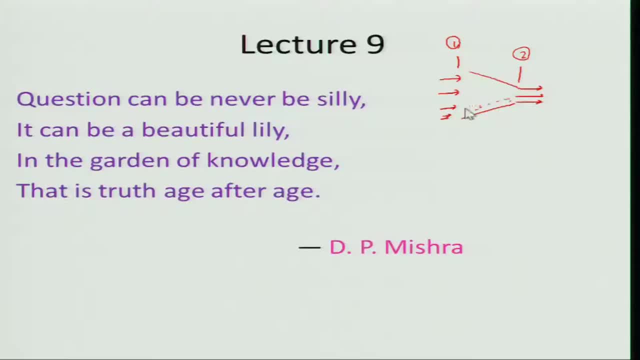 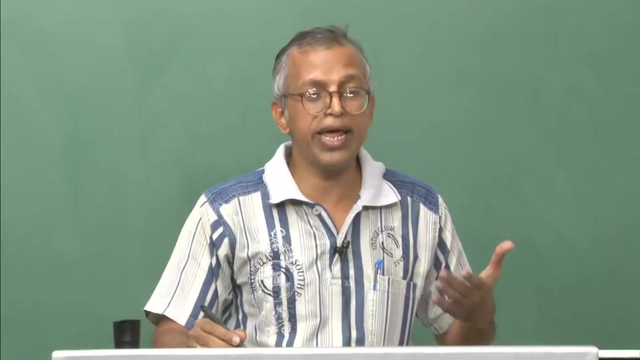 So I have drawn a very, very thin one, but it is very, very thin right. If I just remove it, you know, you will see that it will be in very, very thin right and where there is a likelihood of friction will be playing a role because of boundary layer. 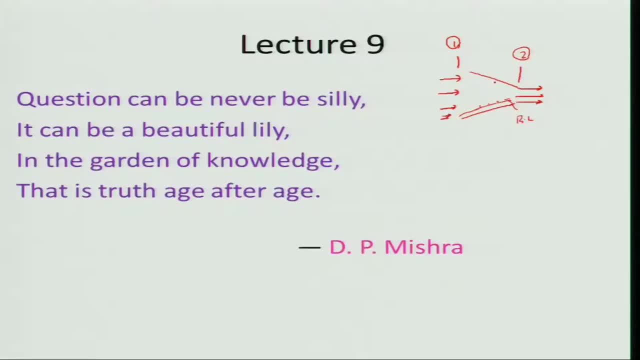 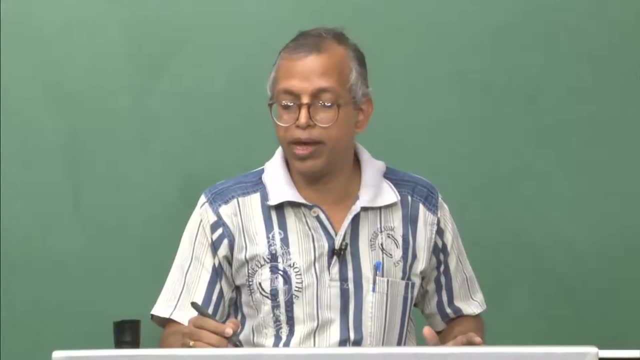 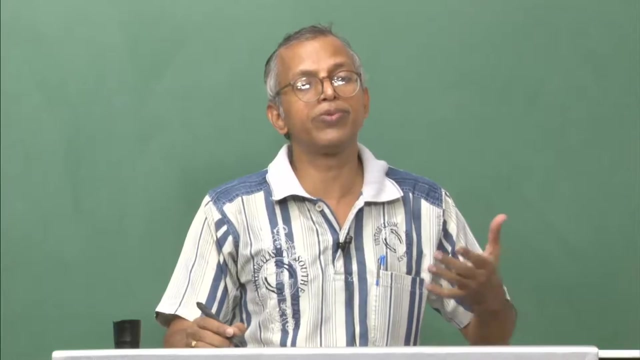 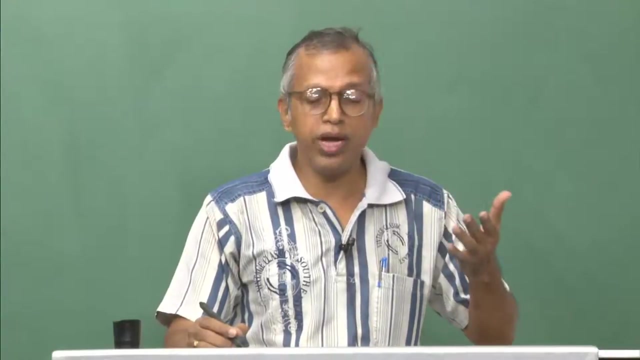 because of boundary layer and also on the upper surface because it is circular. So it is on the over the internal surface surface area. it will be there And whereas inside this flow, whatever, inside it will be not subjected to any what change in entropy? because we are assuming the flow is to be. 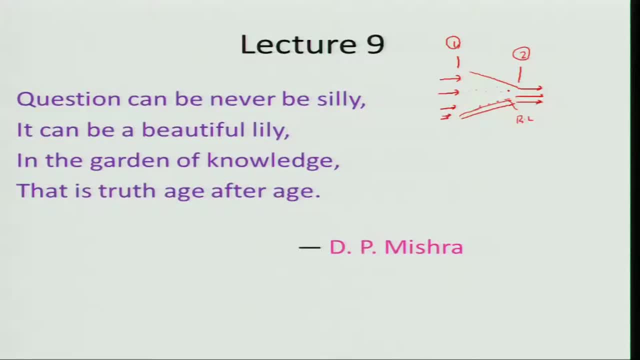 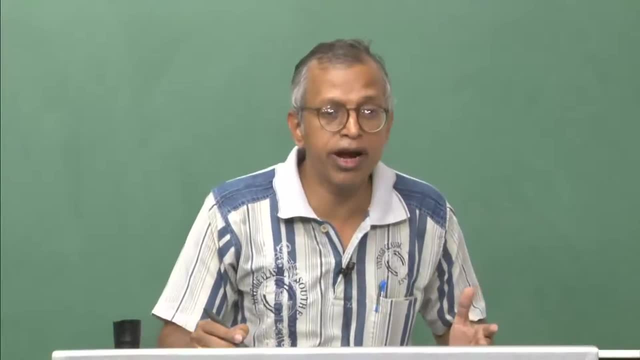 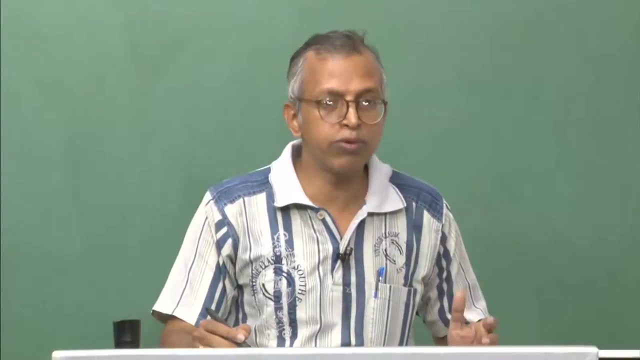 uniform right And also there is no gradient is occurring for entropy to occur, particularly if, look at, there is no temperature gradient, we are not adding any heat right or we are not having any diffusion- mass diffusion- where the entropy can also change because of mixings. 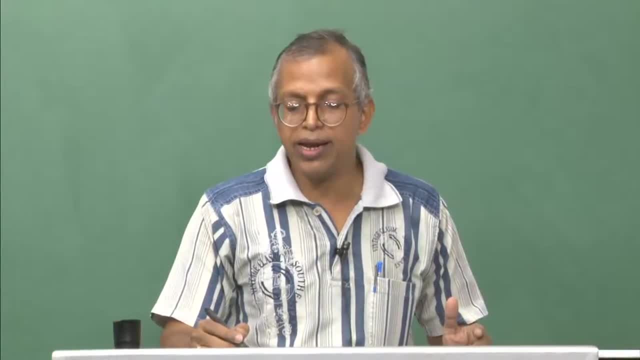 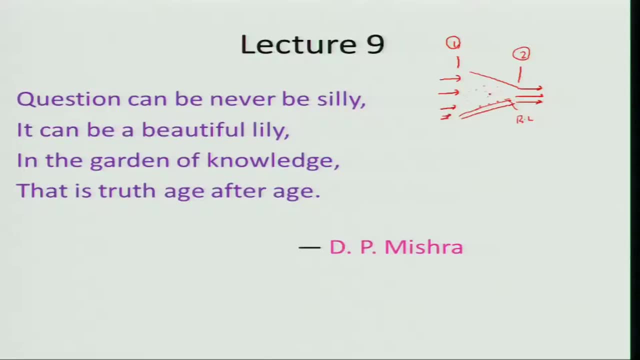 right and then naturally we are not adding heat, So it will be adiabatic, So there is no dissipation in the major region of the flow. then we can consider the flow to be isentropic in the major portion of the flow, except near in this boundary layer which is a very thin 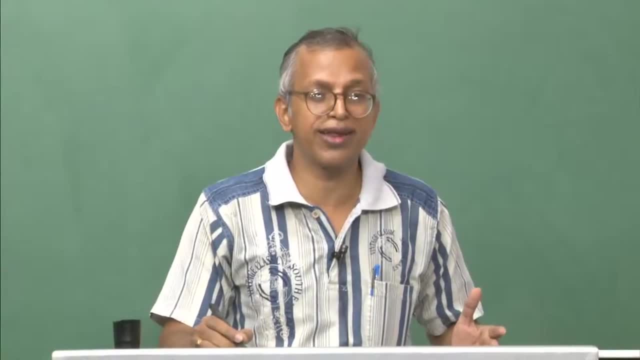 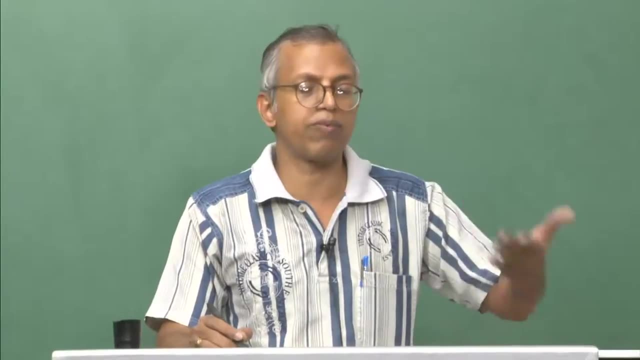 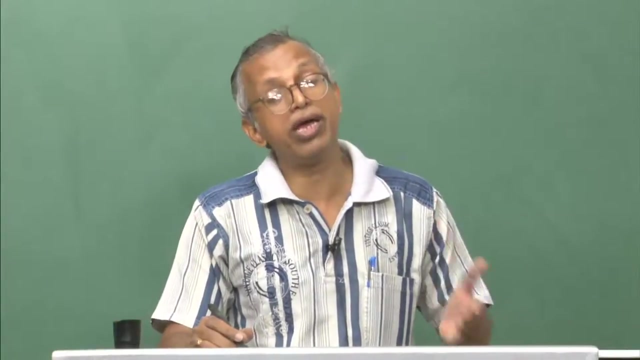 what will be the thickness of the boundary layer? it will be order of few mm. of course, that depends upon inlet Reynolds numbers, and up to talk about are the fluid velocities. as it is accelerating, it will be very small as compared to a decelerating flow. So therefore, 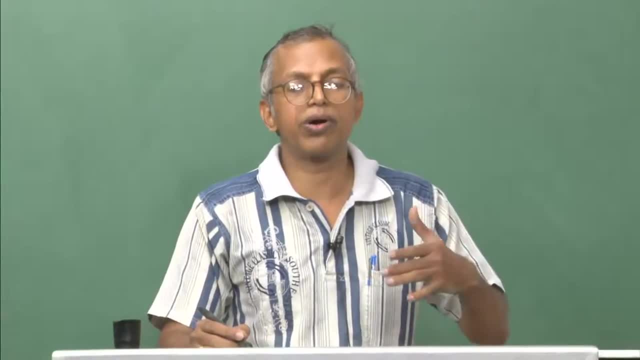 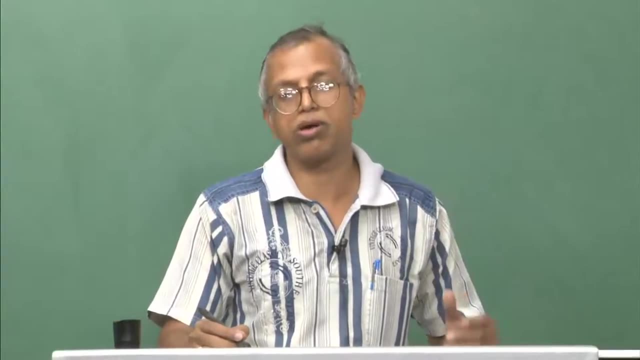 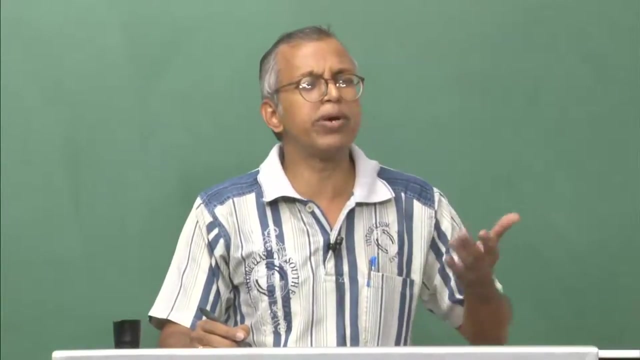 most of the propulsive devices are what you call can be consider propulsive devices like rocket nozzles or a diffusers or a, you know, even turbine blade flow through the turbine compressor. to some extent we can consider it to be an isentropic and carry out, you know. 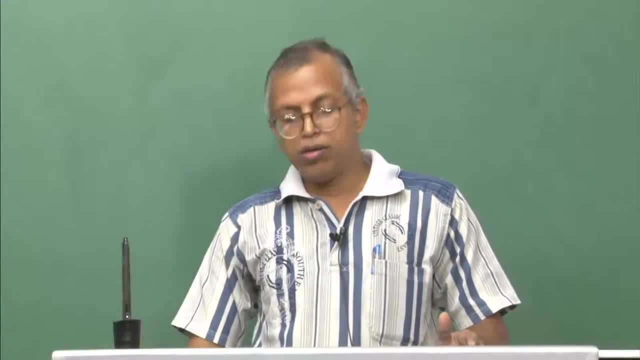 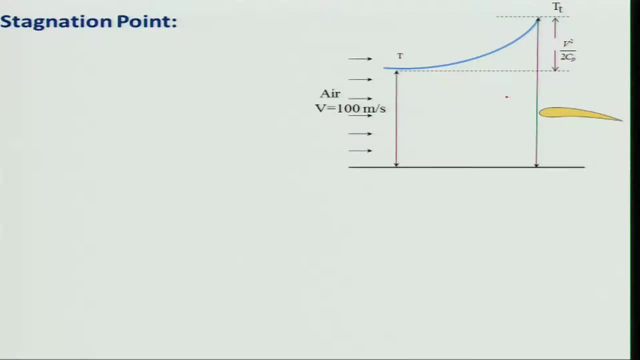 analysis for that. So there is another concept, what we are we would like to look at, which is the stagnation point, what you mean by this stagnation point? let us consider a flow over an aerofoil. I have shown aerofoil here and flow is coming. 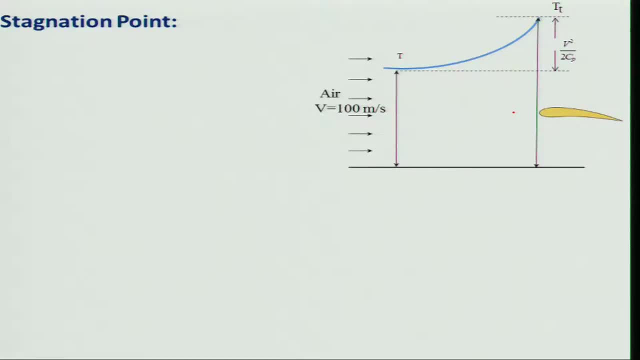 uniform velocity, little away from the aerofoil, and keep in mind that air is flowing over this aerofoil right at a velocity- inlet velocity or upstream velocity- of 100 meter per second. Now, if this fluid you know will be taking, it will be going in a stream line kind of 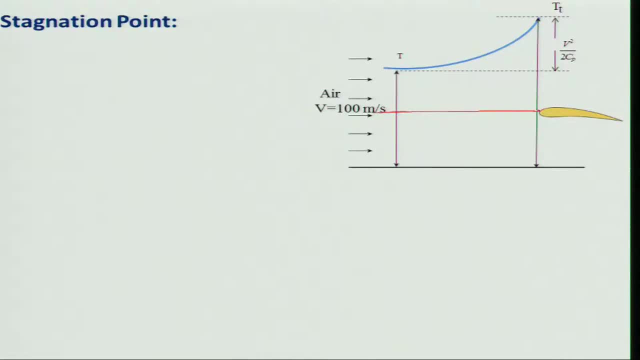 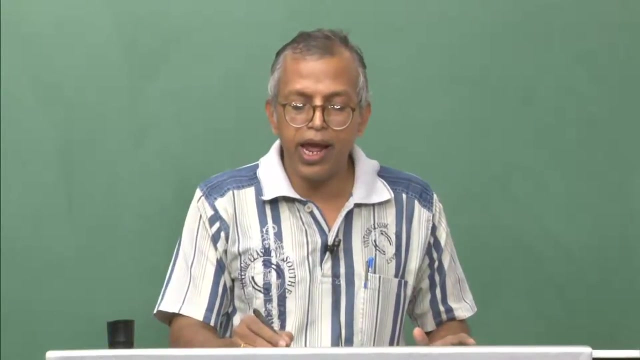 thing: if I take this fluid velocity over here, if you look at the leading edge, it will come to a what you call stand still, right. So fluid element as brought to 0 velocity, right, and if I take, of course, somewhere here, then fluid will go over like this and So 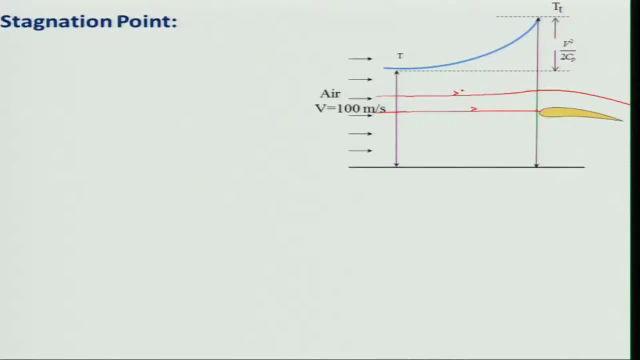 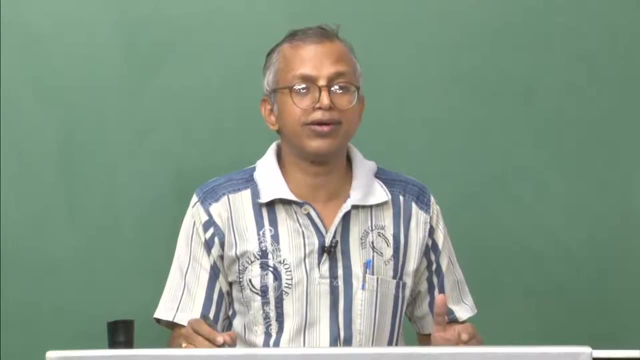 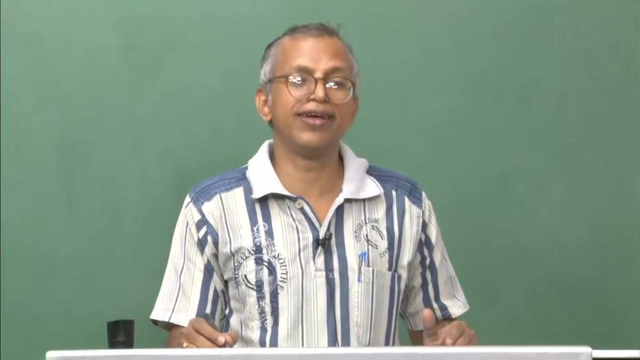 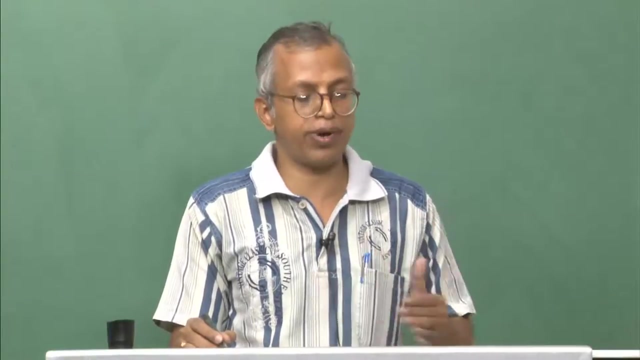 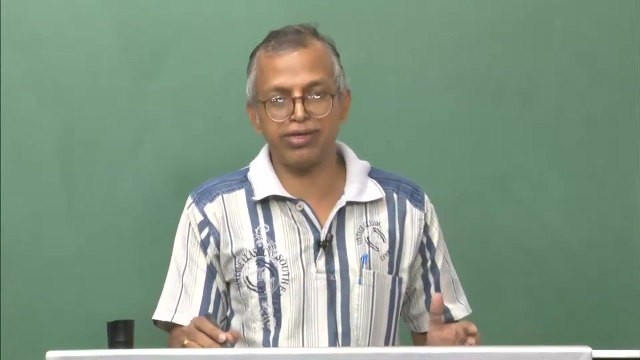 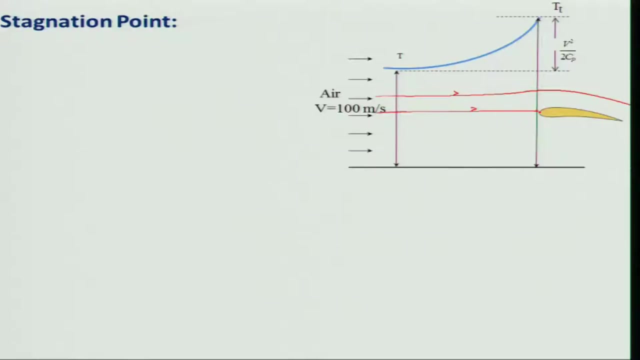 similarly on the lower region. another thing: and now, when this is brought to the 0 velocity right adiabatically and also reversibly, then we call it as an isentropic. that means, if the fluid element is brought Adiabatically to the 0 velocity, then we call it as a stagnation point or a stagnation properties. 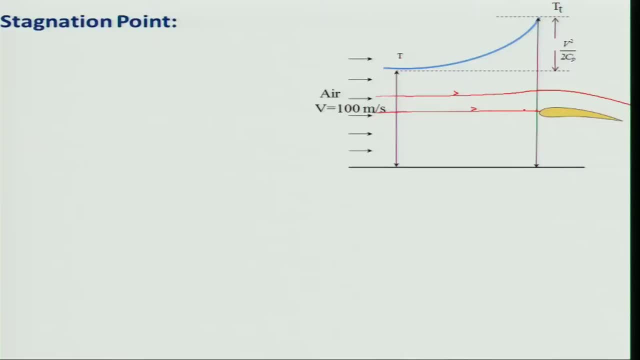 that means, if I am considering as a pressure, it will be. you know fluid experience, you know like fluid will be stagnation pressure. and if I apply, under this condition, the first law of thermodynamics Right, that is the energy equation that we can s? t is equal to h plus v square by 2. what 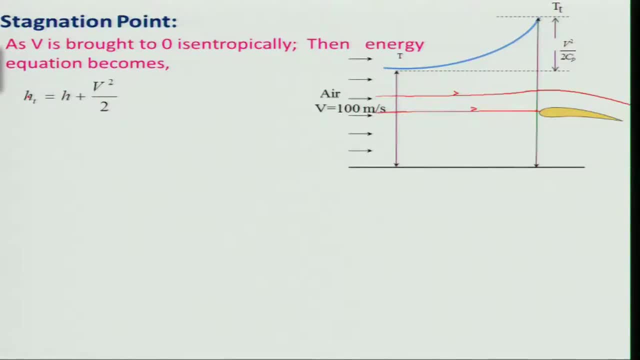 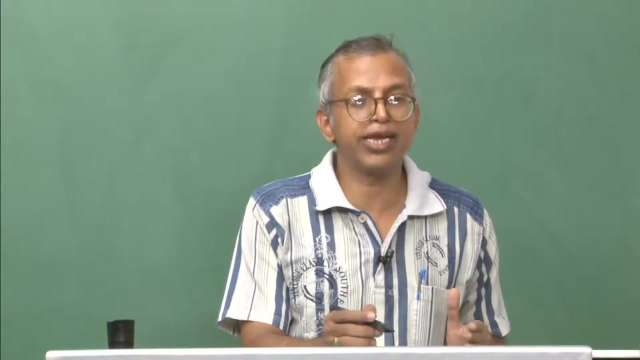 it indicates. it indicates the total enthalpy is equal to the static enthalpy plus v square by 2. right, that is your dynamic energy right And, if I assume, calorifically perfect gas. that means what the C? p is, not a function of temperature in. 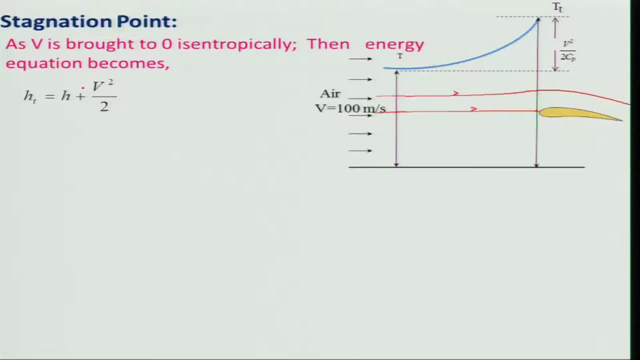 this case that means H will be basically C p t, that is your calorifically perfect gas. then I can write down that T t is equal to T plus V square by 2 C p. What I am doing I am by definition. I am saying H is equal to C p t and then putting it here, that is. 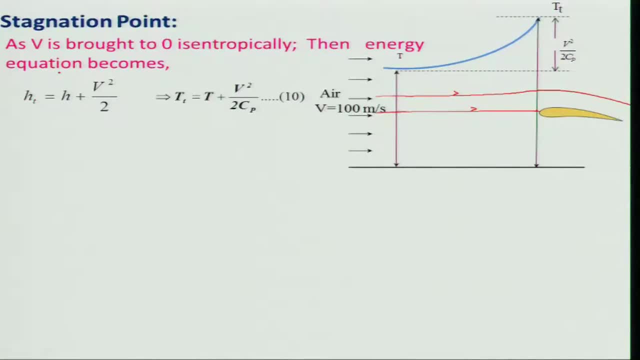 a total, and then here also it will be what you call C p, t, and then if I divide it, then across this, both the left and right and side, I will get T. t is equal to T plus V square by 2 C p. So what is this term? 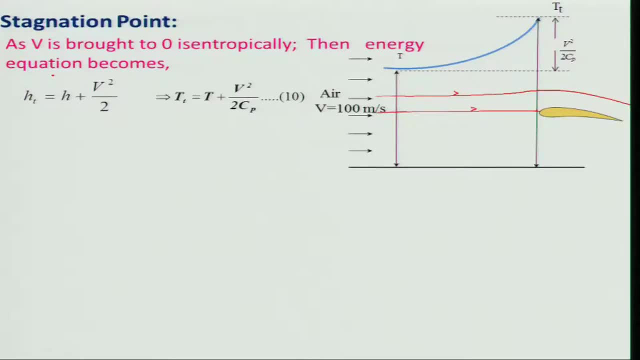 So we call it as a T, this one we call it as a, this term we call it as a static temperature, and this T, t we call it as a total or stagnation temperature, and V square by 2 C p we call it as a dynamic temperature. What do you mean by this static temperature? can anybody tell? 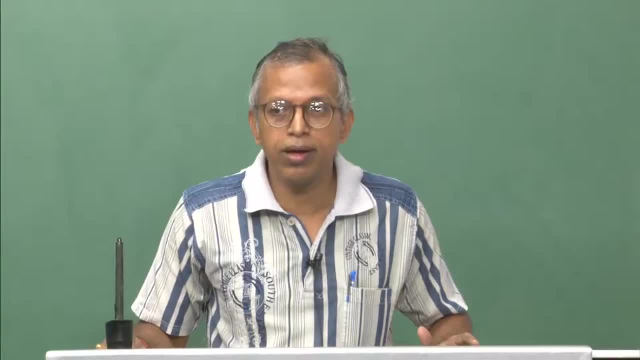 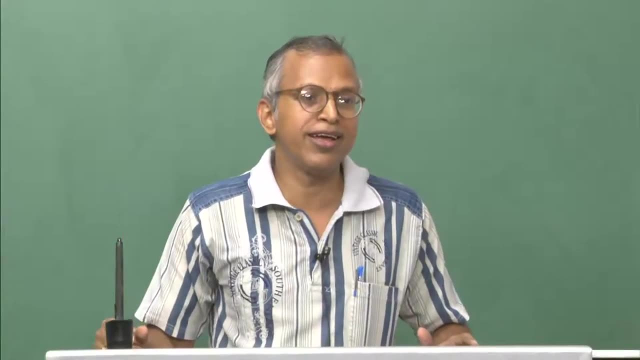 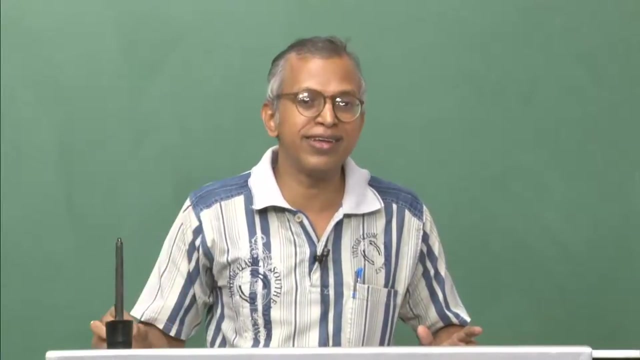 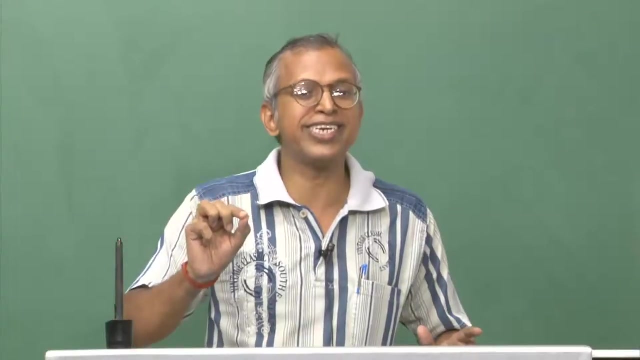 me, That means when the the temperature experience by the fluid element can be termed as a static temperature. in other words, if I put a sensor on the top of a fluid element right which is moving at the local velocity right, what it will be experiencing? it will be experiencing. 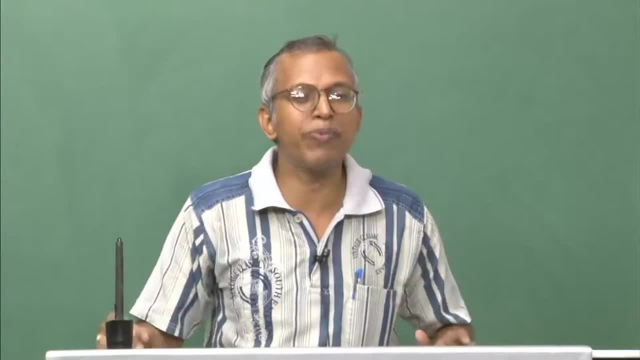 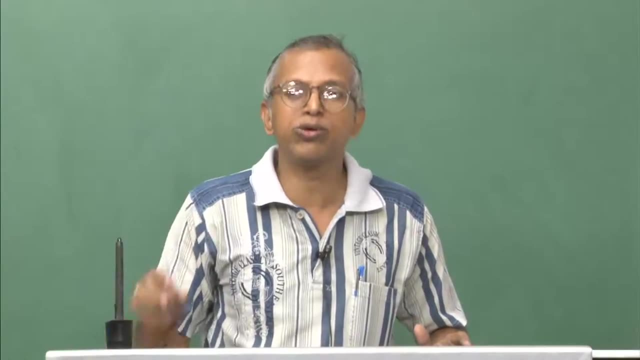 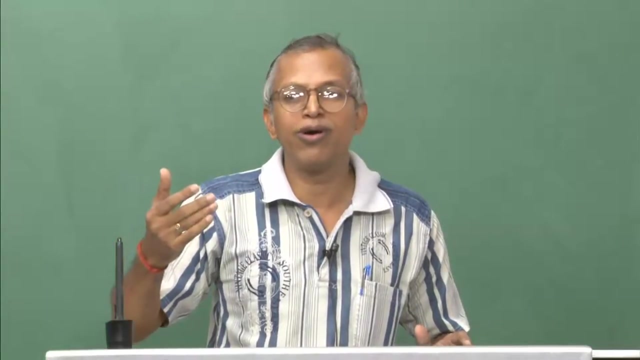 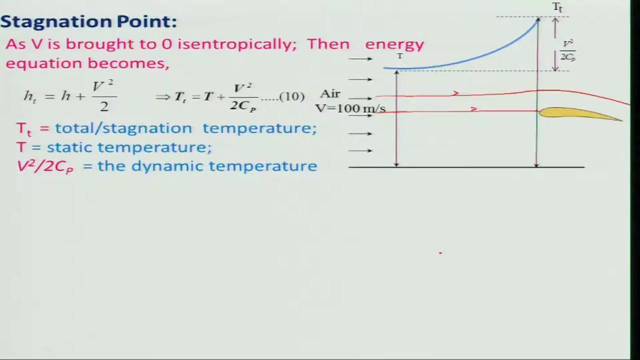 the bombardment of the molecules on the top of it. that is basically the temperature, that kinetic energy, what it will be experiencing. So that is known as static temperature, and as it is moving at a certain velocity, So therefore that velocity will be nothing but v square by 2 C. p is basically the dynamic temperature. 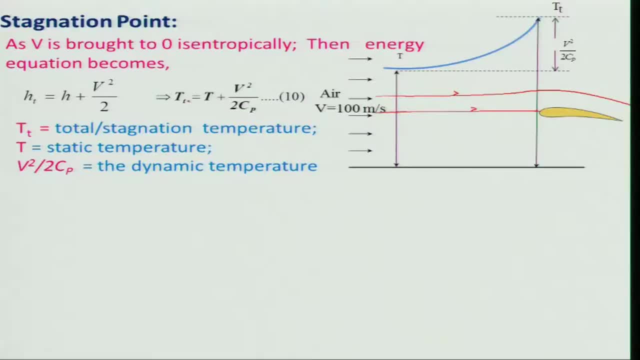 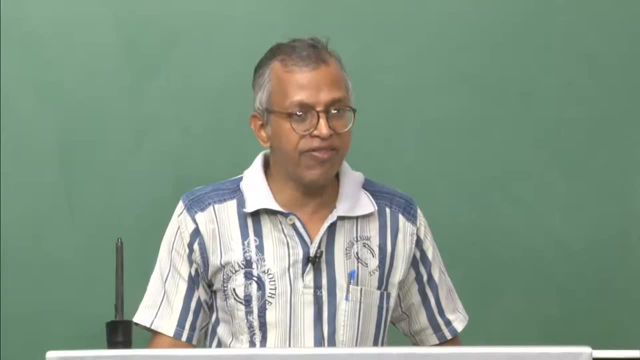 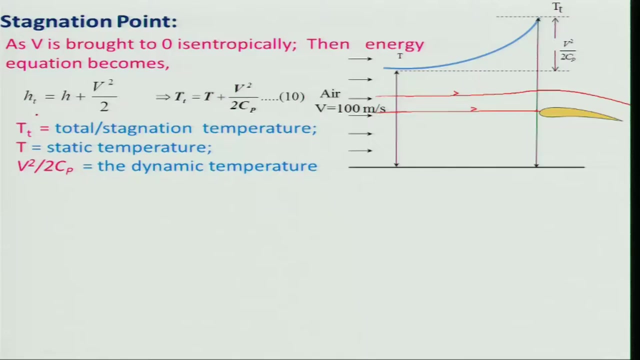 So, and if you look at similarly, we can define also the total pressure. total, you know, density like that, are you getting my point? So what is this meaning? this equation, if you look at S, t is equal to h plus v square by 2. what is saying that means? if I take a station one, 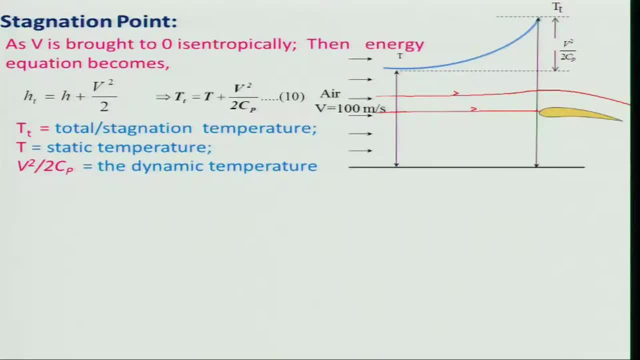 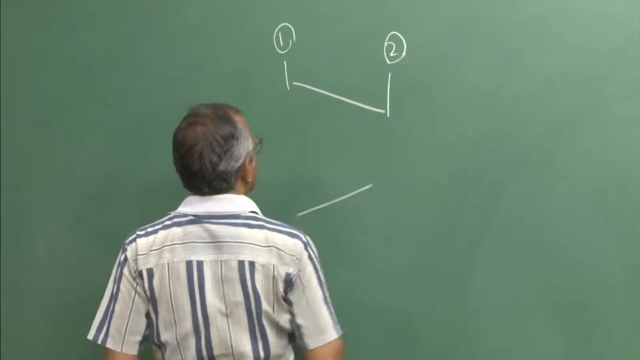 if it, I would take a particular station. You know, Let us say one and the station two, then what I will get right? for example, I am looking at a nozzle, like kind of things. you know, if I am taking this is the one, this is two, right? 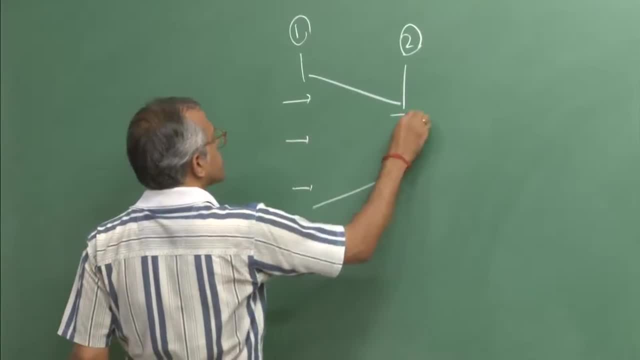 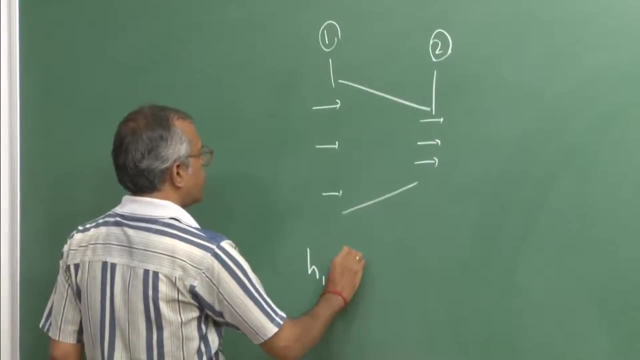 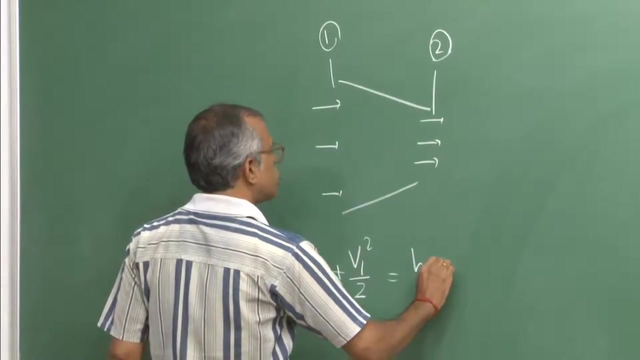 station and there is a flow which is occurring right. If I look at, this is the one, this is the one which is happening right. And then I can write down: h 1 plus v 1 square divided by 2, is equal to. I can write down: h 2 plus v 2 square by 2. that means and is equal to: 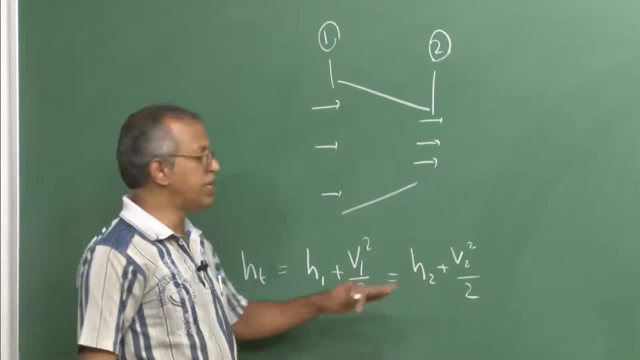 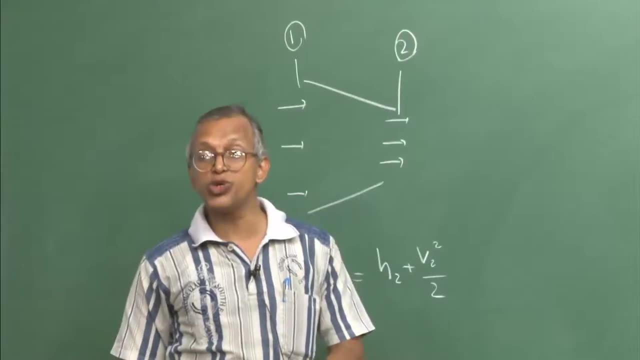 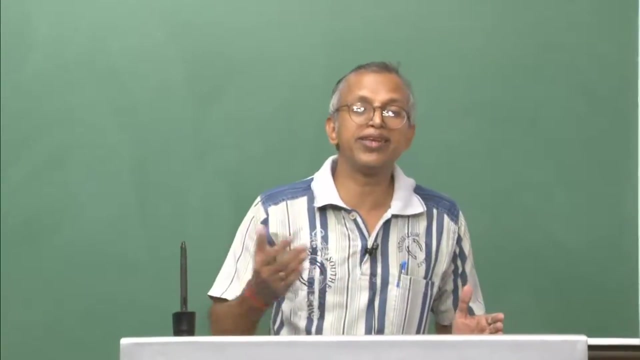 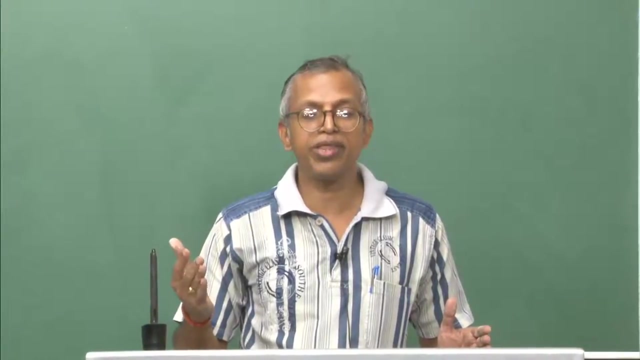 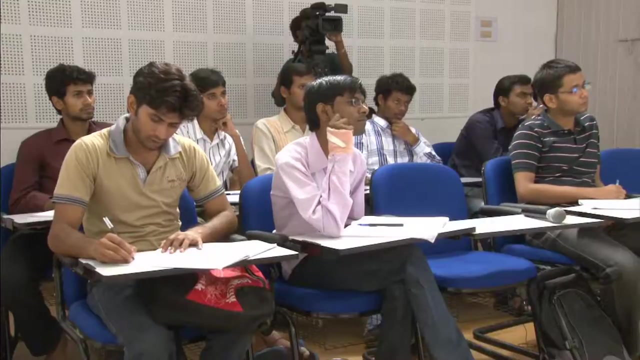 h t. can I say this? that means what is saying: the total enthalpy is remaining same between the station one and station two, right. So That means total enthalpy is remaining same provided the flow is steady, and whether it will be inviscid or not, it will be inviscid then. only is it so, but so far. energy equation. 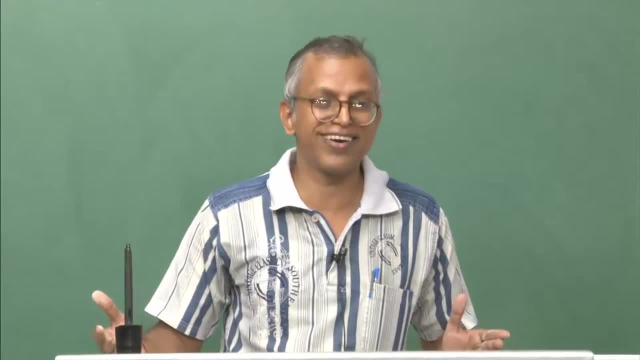 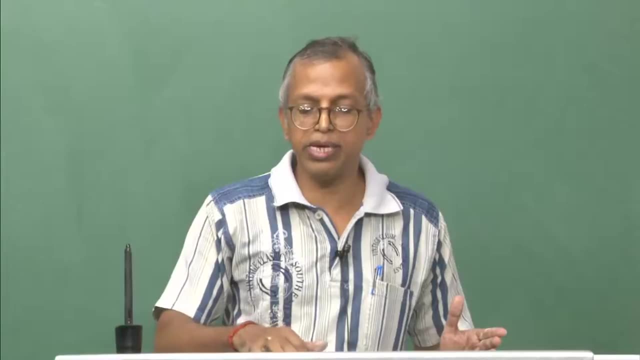 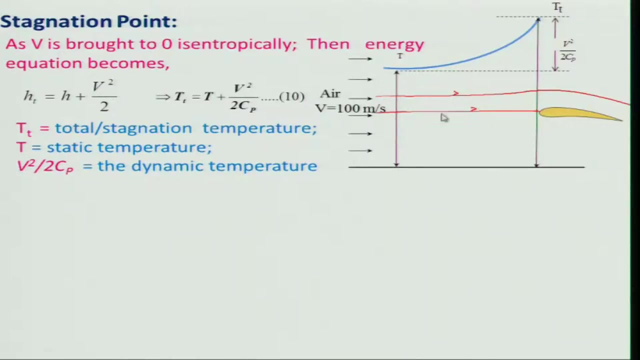 is concerned, we are not worried about whether it is inviscid or not. And then if it happens to be, you know like that means total enthalpy along a stream line remain constant. If it is uniform velocity at the upstream region. that means I can say that along with any 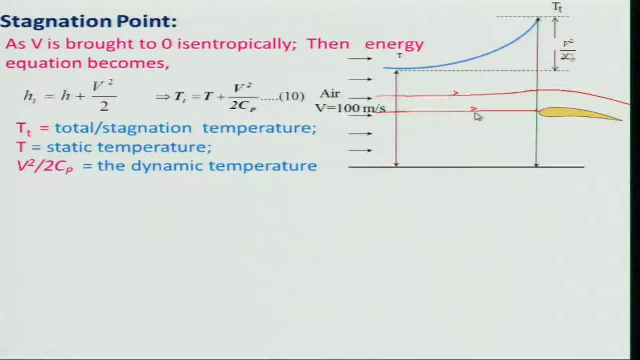 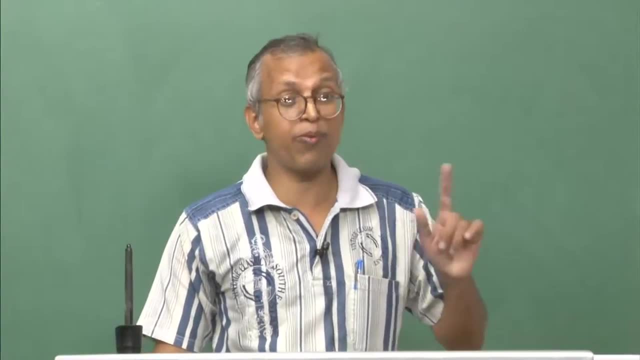 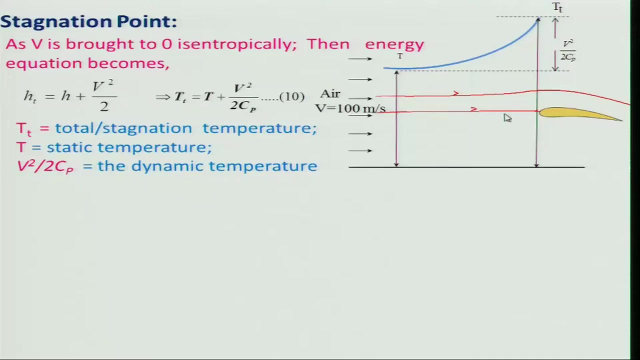 stream line, the total enthalpy remain constant. That means along the whole domain the total enthalpy will be remaining constant, provided the flow is steady Right And it need not to be one dimensional right, because my stream line can be two dimensional. 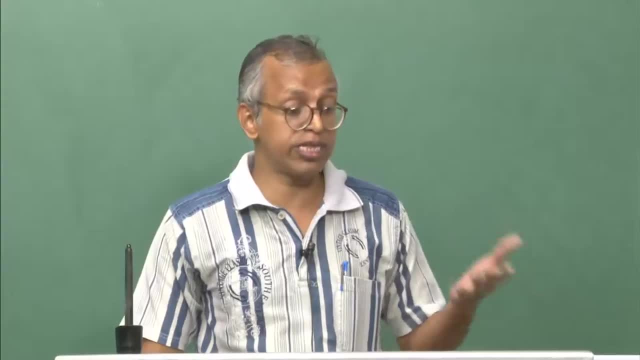 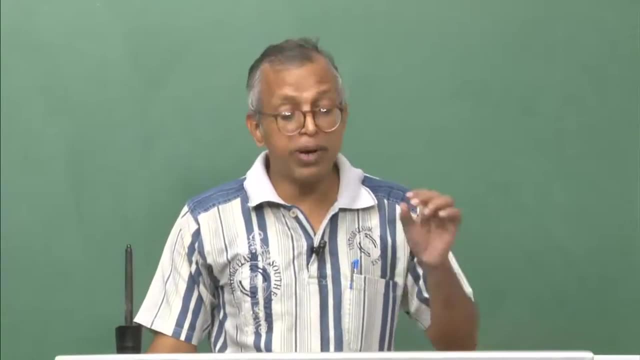 as well, right, So therefore it need not to be one. this is the profound statement. you may see, we have derived for one dimensional flow. now we are talking, but you can interpret that, But keep in mind that total temperature, total pressure, is it really one dimensional? 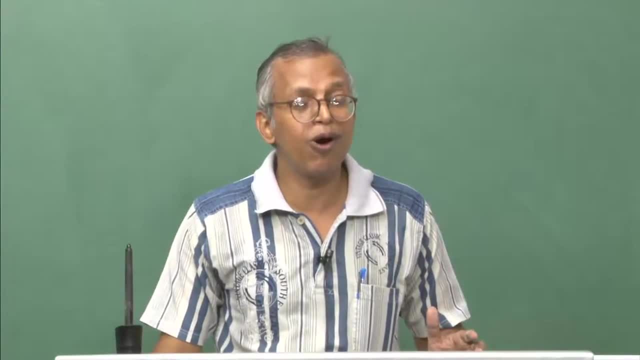 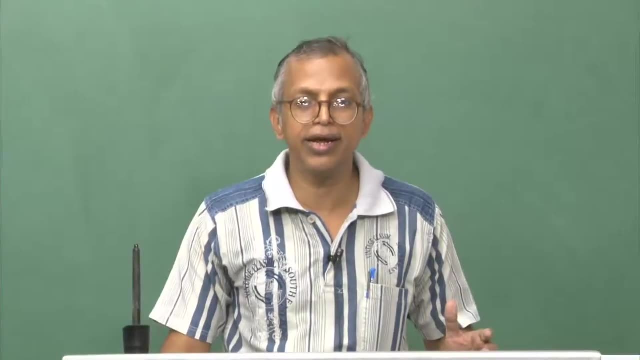 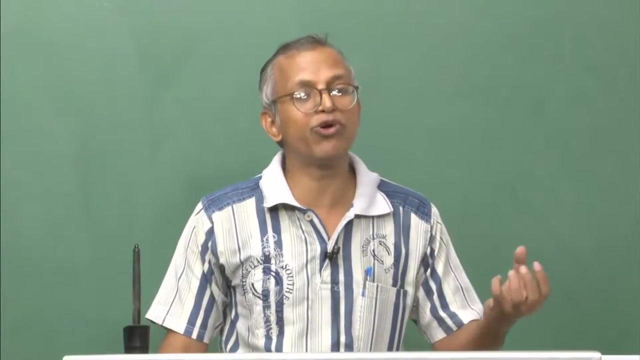 flow. is it really a quantity which you can measure or what is the so big about it? we are talking. It is actually derived quantities, right? And you? it is quite difficult to measure as such, right, because you need to bring the fluid isentropic right. 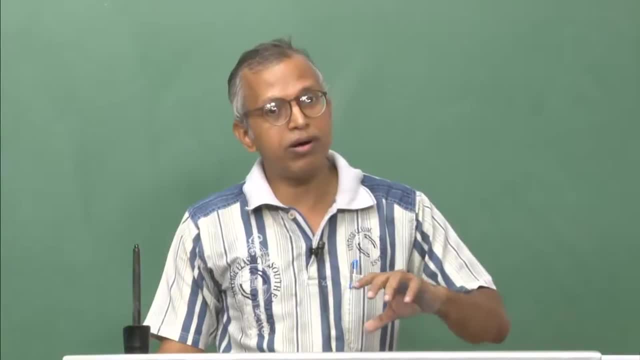 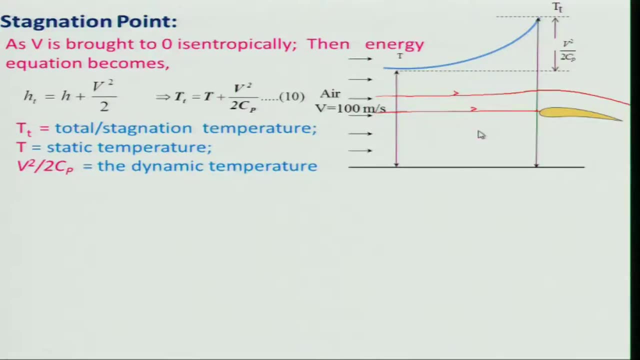 So, therefore, but however you know, at two location the flow need not to be isentropic. However, we can use this relation locally. that is very important point. So I have already talked about this. like T, t represent the temperature and ideal gas attains when it is brought to. 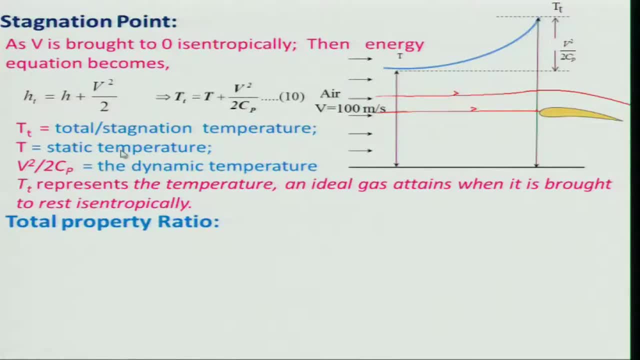 rest isentropically. And having said this, you know about this stagnation point properties. let us look at the total property ratios and that is equation 10 became like this what I will do: I will just divide this T t by the T temperature and also the right hand side. 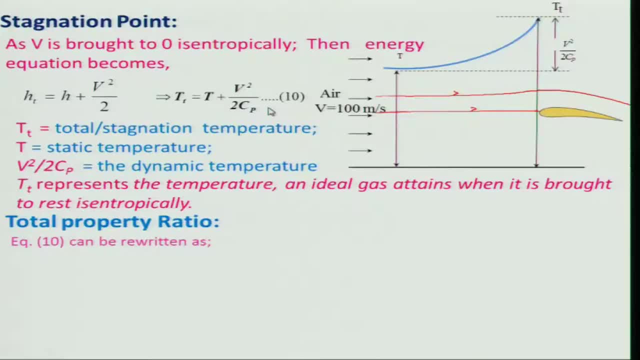 of this equation by the static temperature, T. So what I will get, I will get T. t by T is equal to 1 plus V, square divided by 2. C, p, t, And for a calorific perfect gas, I can write down, you know that is C, p is equal to gamma.